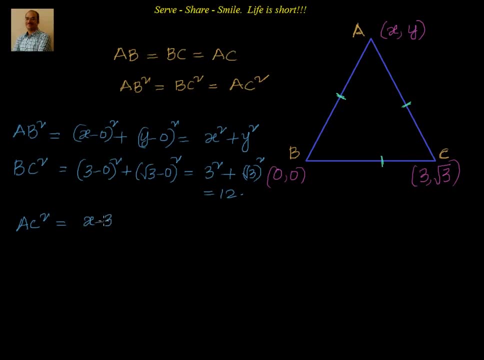 a and c. Can I say x minus 3 whole square, plus y minus root 3 whole square, This is AC square. So we will equate two at a time and our first: we will say that AB square is equal to AC square. That will give us one condition. The other condition we will use is we will say that AB square is equal to BC square. 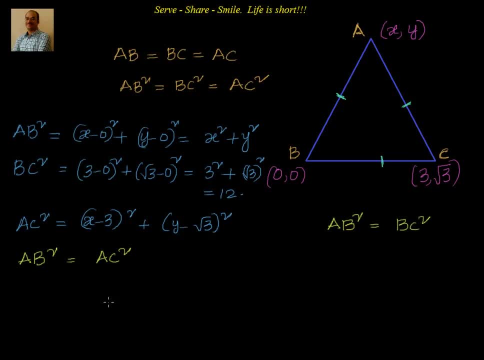 So first we will try to use AB square equal to AC square and try to get a relation between x and y, which we are going to substitute in AB square equal to BC square, and get the values of x and y. So what is AB square? We know x square plus y square. So let me write it down: x square plus y square is equal to x minus 3 whole square. 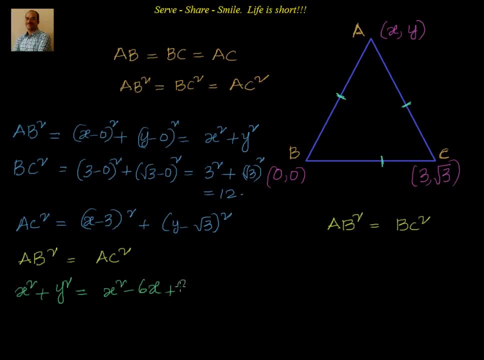 Let us open it up: x square minus 6x plus 9 plus y square minus 2 root 3, y plus 3.. So we have AB square equal to AC square. So can I cancel x square plus y square on both the sides I will have. if I take 6x and 2 root 3 y to that side, I will have 6x plus 2 root 3, y is equal to 12.. 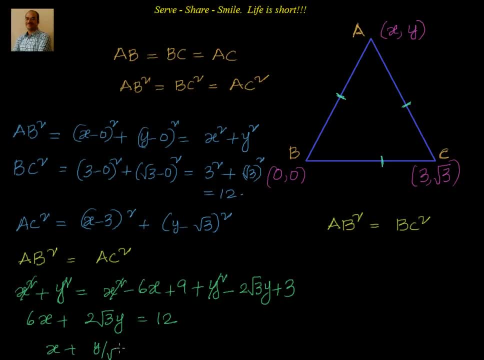 If I divide by 6, I will have x plus y by root 3 equal to 2.. So we divided by 6. 6 into x, 2, root 3 by 6.. 2 will go 3 times. Root 3 by 3 is 1 by root 3. 6 will go 2 times. 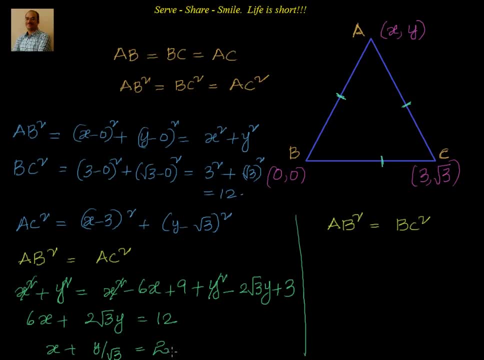 Now what we will do This: x plus y. by root, 3 equal to 2. whatever we have conditioned from that, we will get y and we will substitute it in terms of x. So my next step will be: We will write down: AB square, x square plus y square is equal to BC square, that is, equal to 12.. 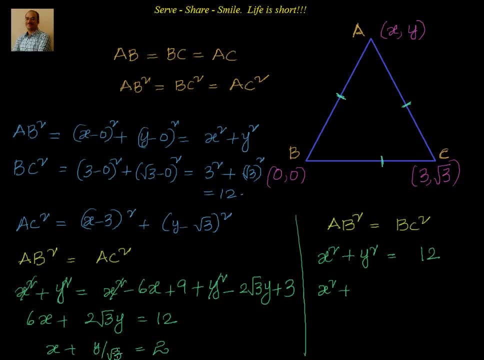 Now x square plus instead of y, I want to write down y in terms of x. So can I say y equal to root 3 into 2 minus x. We should be okay with that, because y by root 3 is 2 minus x. 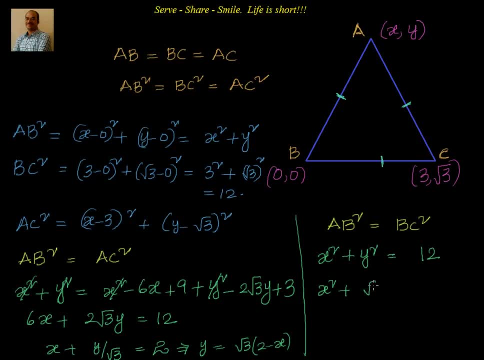 So I can substitute here. I will have root 3 whole square into 2 minus x whole square, equal to 12.. If we open this up, we will have x square plus 3 into 2 minus x whole square, Or can I say 3 into x minus 2 whole square, equal to 12.. 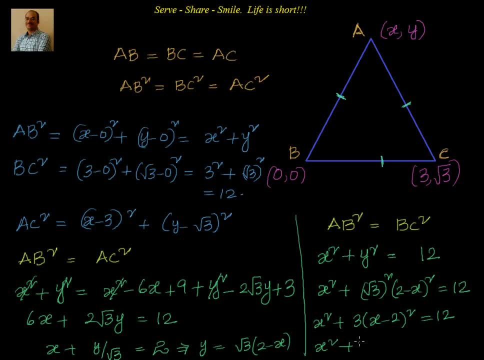 So we will open up x square plus 3 into x square minus 4x plus 4.. 4 is equal to 12.. So the next step will be x square plus x square plus 3 into x square, 3x square minus 12x plus 12, equal to 12.. 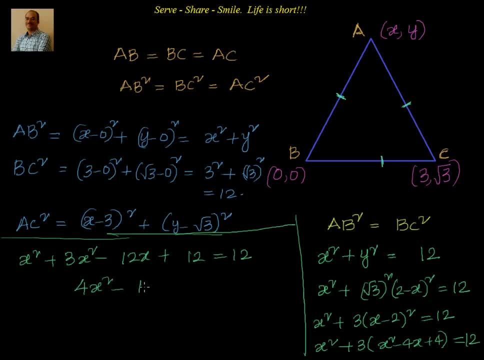 Can I say 4x square minus 12x equal to 12.. 12, 12 cancel equal to 0. or can I say 4x into x minus 3, equal to 0.. Therefore, x equal to 0 or x equal to 3.. 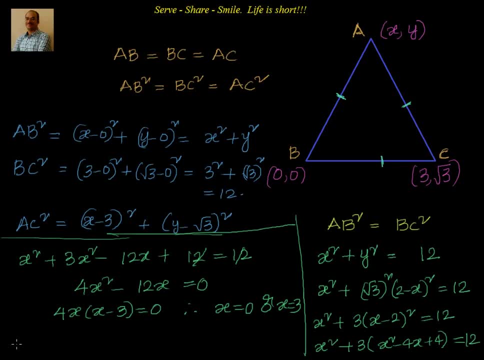 So if x equal to 0, what will be the value? So we will write down that if x equal to 0, put x equal to 0.. Where is our y y equal to? we will write down here what we got y equal to root 3 into. 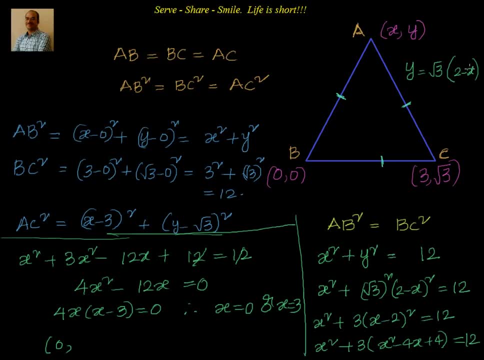 2 minus x. So if I substitute x equal to 0, y will be 2 comma 2 root 3.. That will be one coordinate. The other one will be If I put x equal to 3.. I will have 2 minus 3 minus 1.. 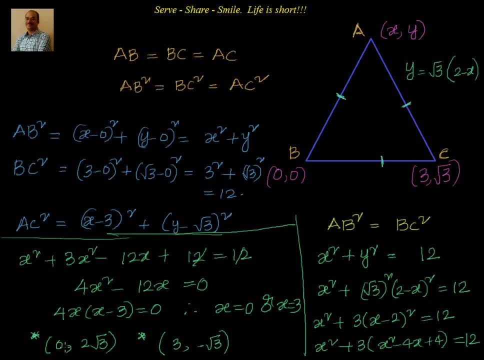 That will be minus root 3.. So the values of x comma y are 0 comma 2 root, 3 comma, 3 comma minus root 3. So why we have 2.. Why we have 2 points? because when it is an equilateral triangle we can have the point on this quadrant or we can also have it in this also. 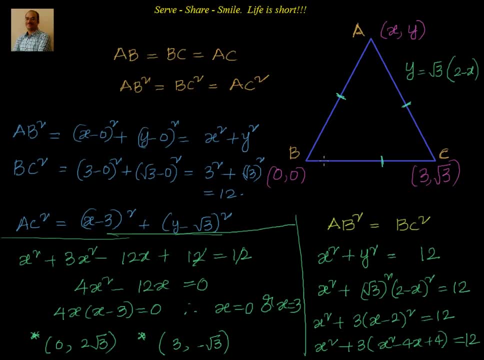 So we can have. we can have a to above of b c, or I can also have a below b c. So we have 2 options. So that is the values of x, comma, y. Let me summarize this: We have been given equilateral triangle. 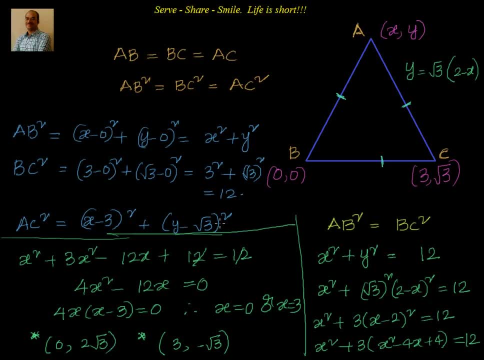 We have been told that We have been given equilateral triangle. The vertices are 0 comma, 0, 3 comma, root 3.. We have to find out the third vertex, Coordinates of the third vertex. So what we have done, We know. equilateral triangle property. 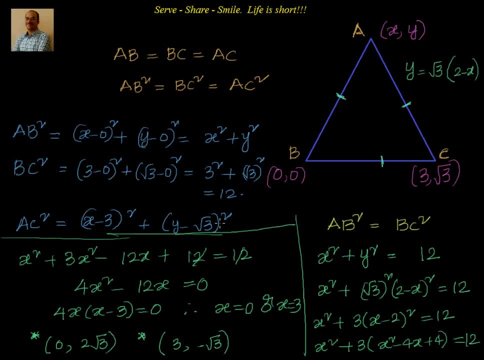 All the sides are equal: a b equal to b c equal to a c Square. it up: a b square equal to b c square equal to a c square. We have written down what is a b square, What is b c square. 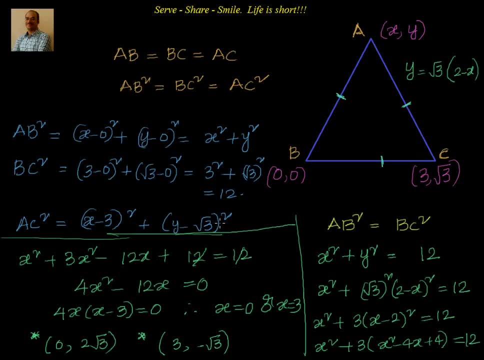 What is a c square? We use it. a b square equal to a c square. We found out a relation between x and y, That y equal to root 3 into 2 minus x. Once we know that We went to a b square, equal to b c square. 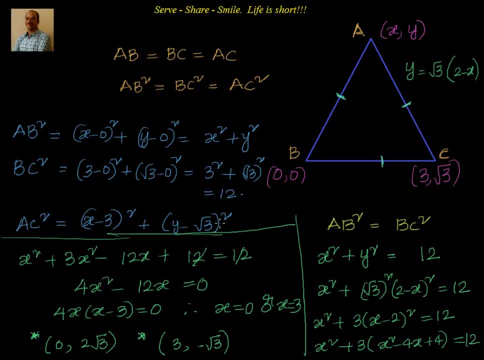 Because on b- c square we have constant term there 12.. So we have converted y in terms of x And solved for linear equation In one variable. it will become And we got 4, x equal to 12 and x equal to 3.. 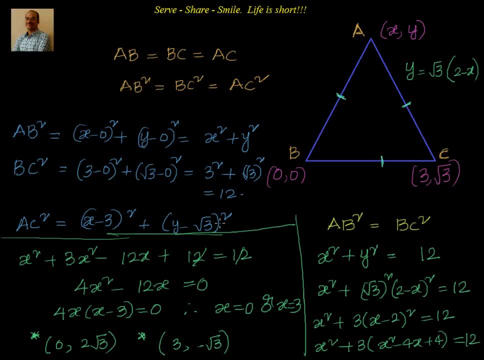 It is actually. We got an quadratic equation Where constant terms are cancelling And we got: We got 4 x square minus 12, x equal to 0. Or I take 4 x common: we got x equal to 0 or x equal to 3.. 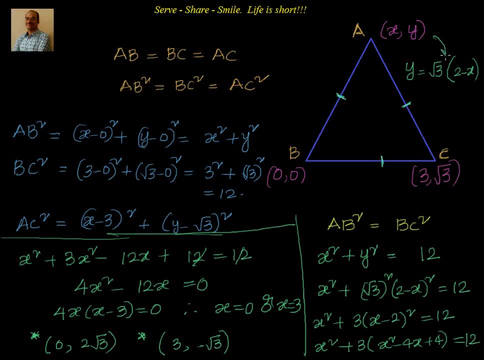 So once we got x equal to 0 or x equal to 3.. We can go back to y equal to root 3, into y equal to root 3 into 2 minus x. Substitute x value: if x equal to 0, y equal to 2 root 3.. 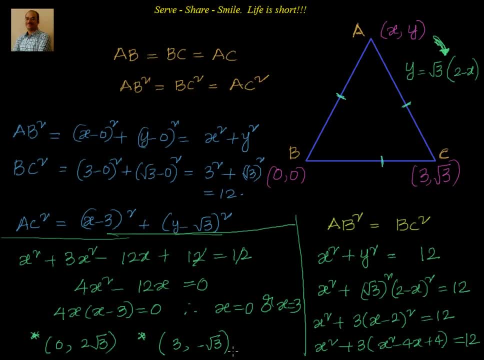 If x equal to 3, y equal to minus root 3.. So that is one interesting example I thought of sharing related to corner geometry, distance between points, How to find, How to find out the third vertex of an equilateral triangle. Thanks for your time and support. Bye for now. 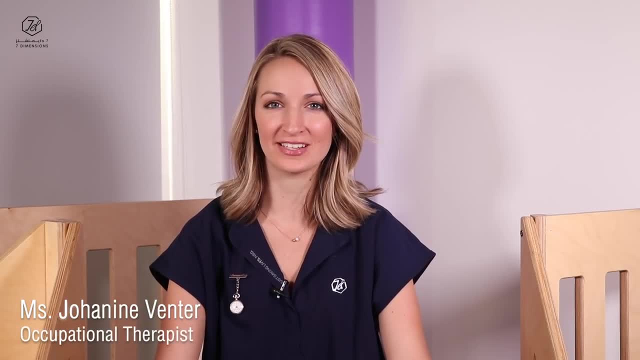 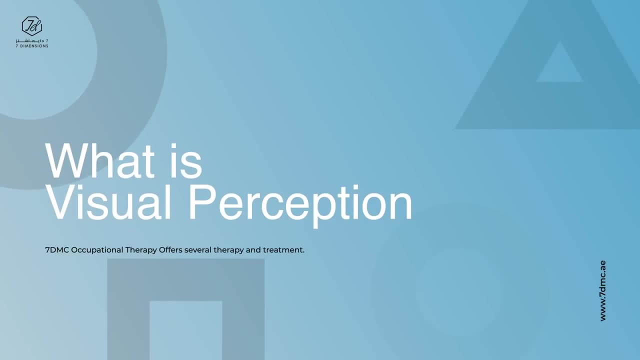 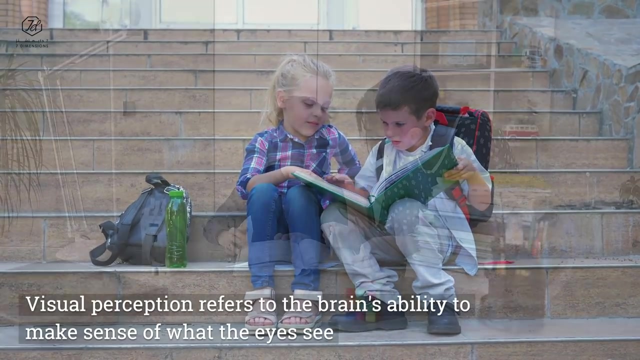 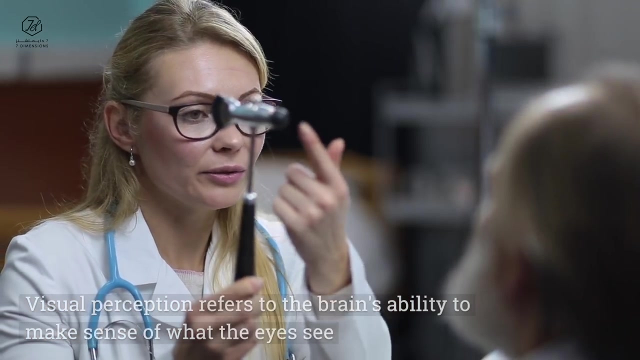 Hi, my name is Ioannine and I'm the Occupational Therapist at Seven Dimensions Medical Centre. Many kids struggle with reading, writing and copying activities, and often this is due to visual problems. However, what do you do when you've done the vision test and everything comes back normal?